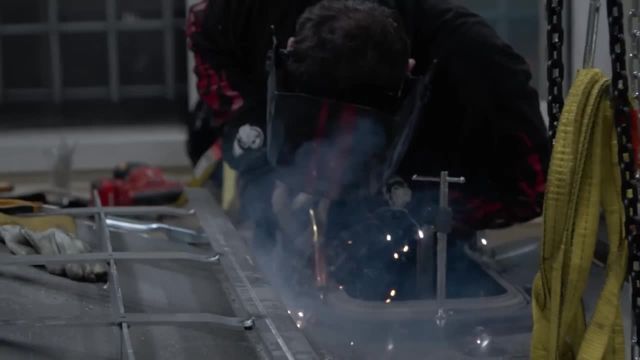 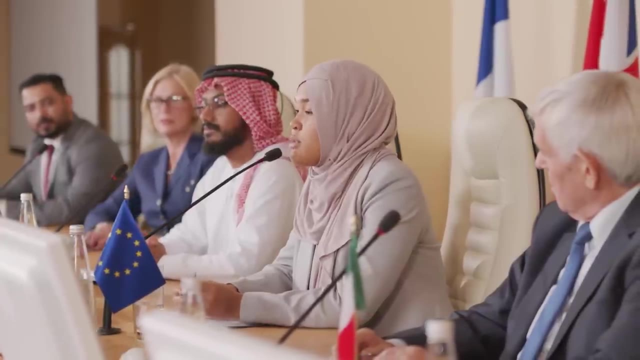 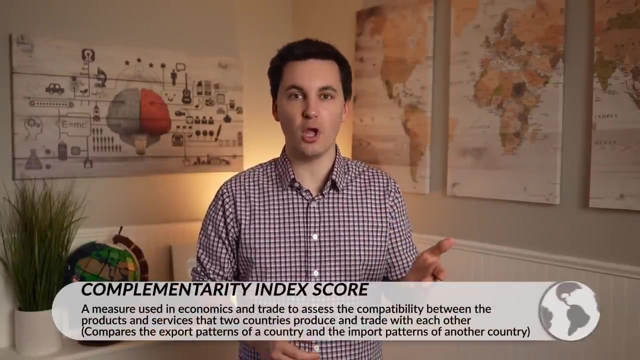 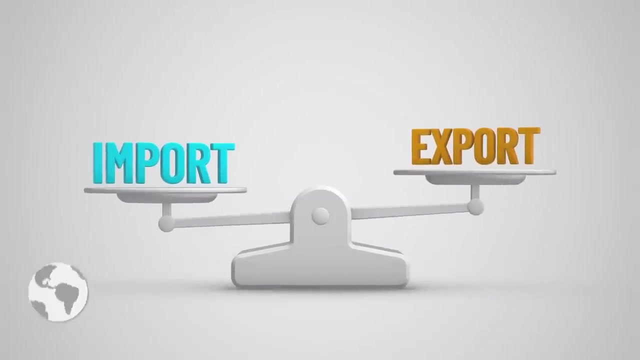 more goods, see improved efficiency and productivity, gain the ability to specialize more, access new technologies and ideas, and can even strengthen their political relationships with other countries. When looking at global trade, we can see that countries that have a stronger trade complementary index score will be more likely to trade with one another. The complementary index compares the export patterns of a country and the import patterns of another country. A higher score indicates a more favorable trade relationship. The complementary index 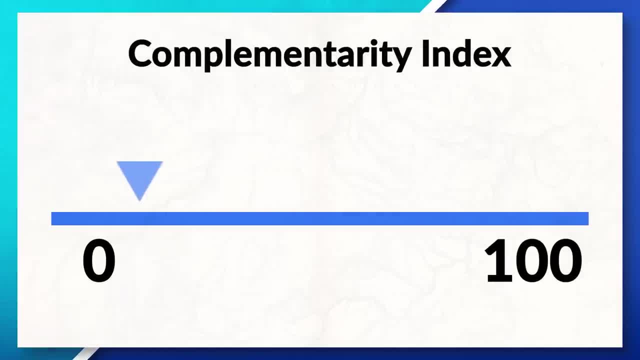 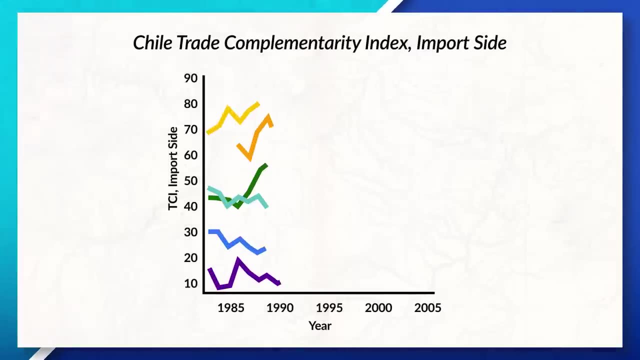 can range anywhere from 0 to 100, with 0 meaning the two countries do not complement each other at all, and a score of 100 meaning the two countries exports and imports perfectly match. For example, we can see here that Chile's imports are more complementary with countries in North America compared to countries that are in Latin America. By looking at this data from the World Trade Organization, we can see that Chile and the United States are the most compatible trade partners, while Bolivia and Peru are the least compatible. So it would make more sense for the 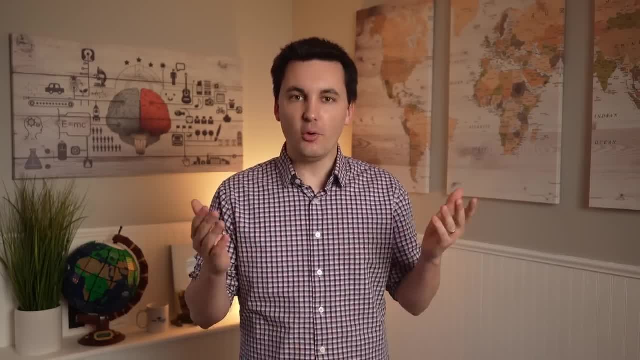 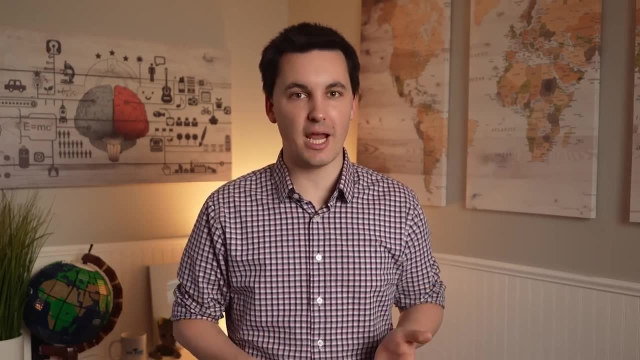 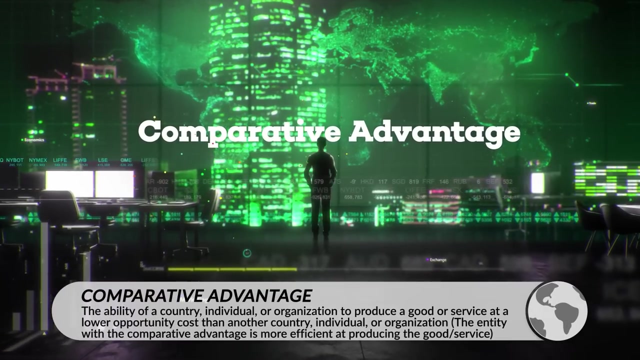 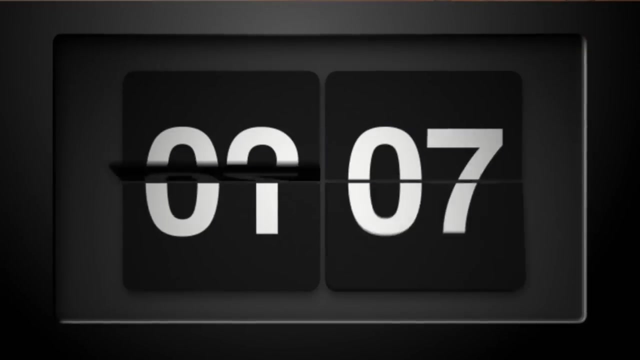 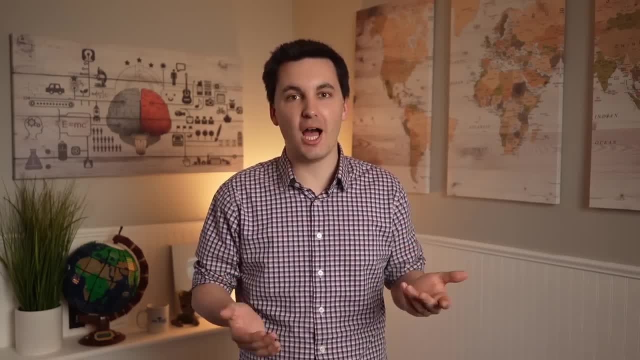 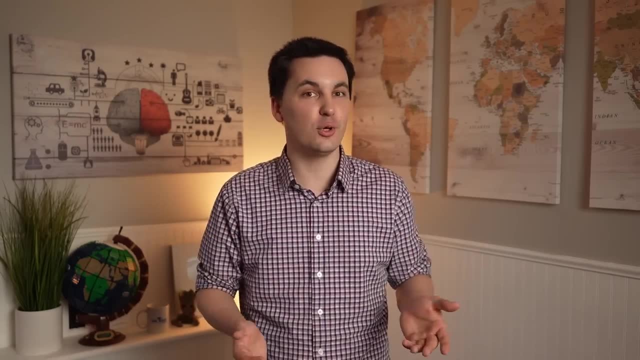 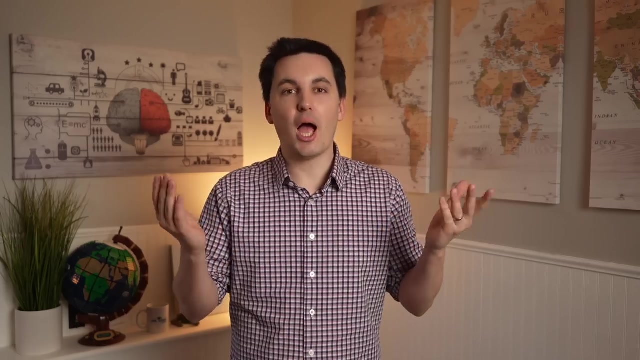 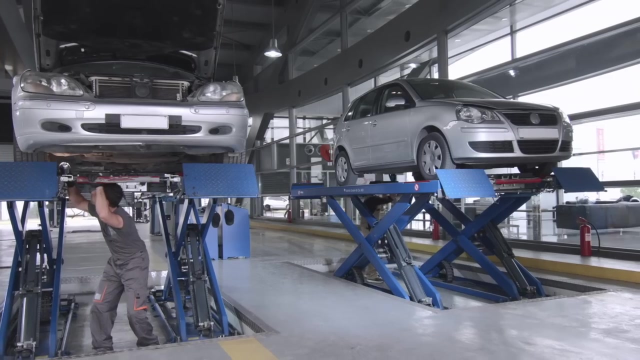 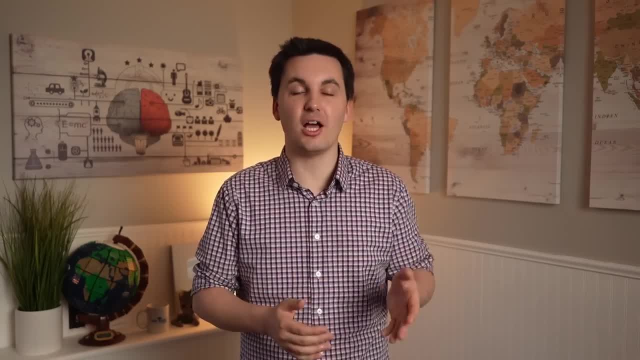 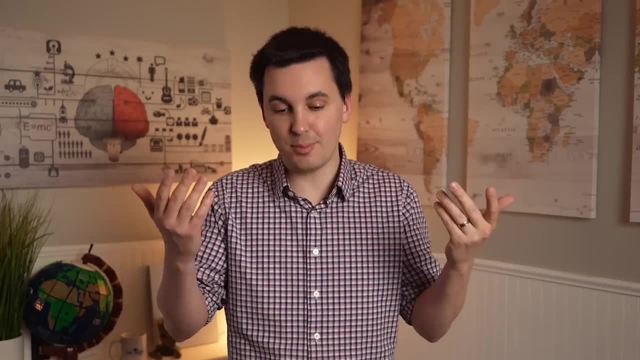 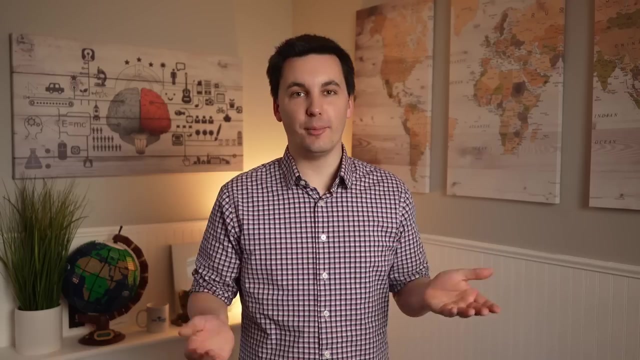 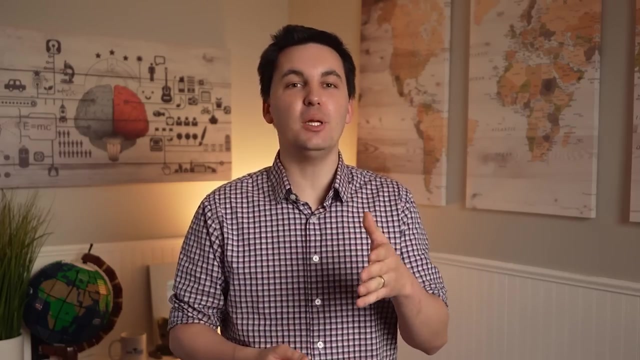 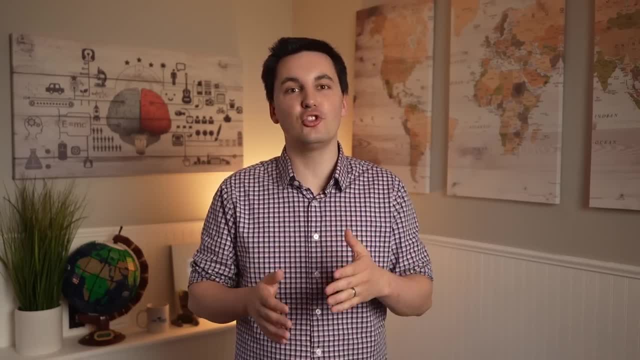 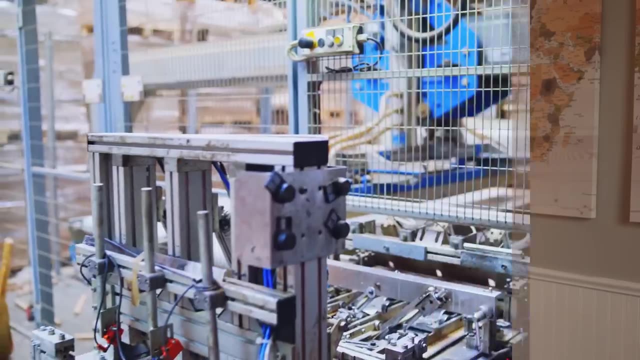 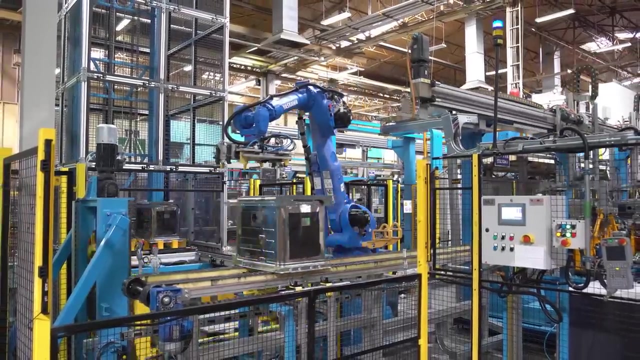 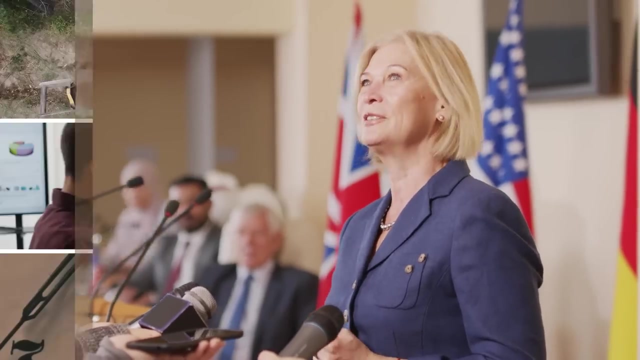 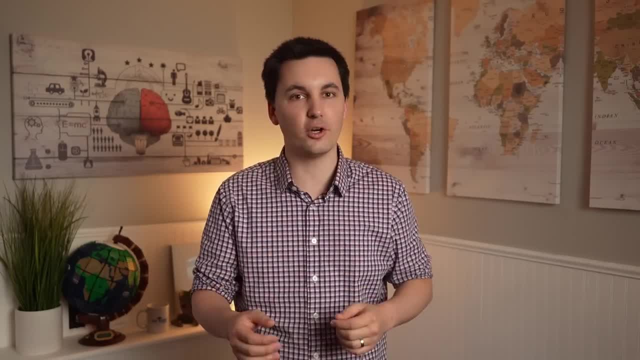 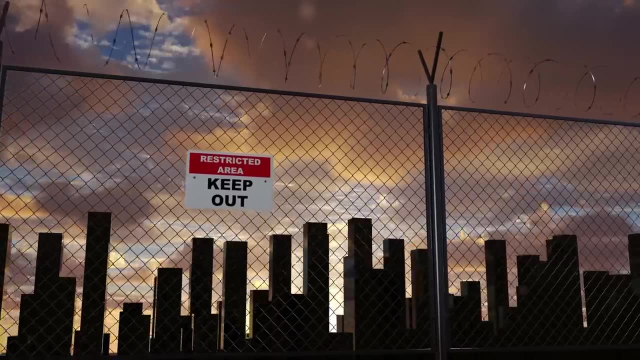 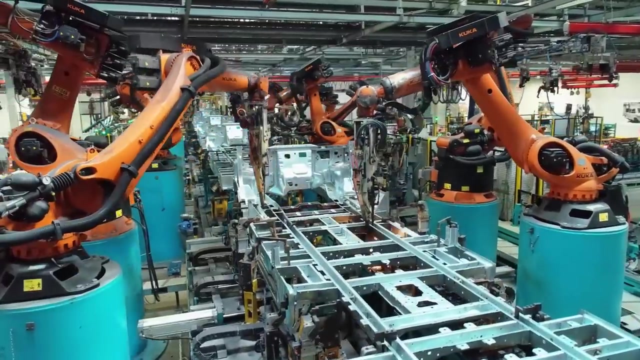 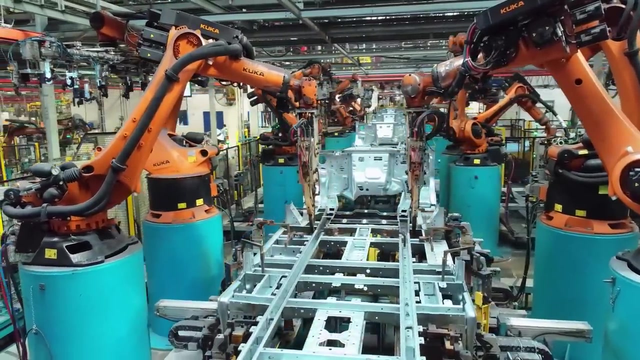 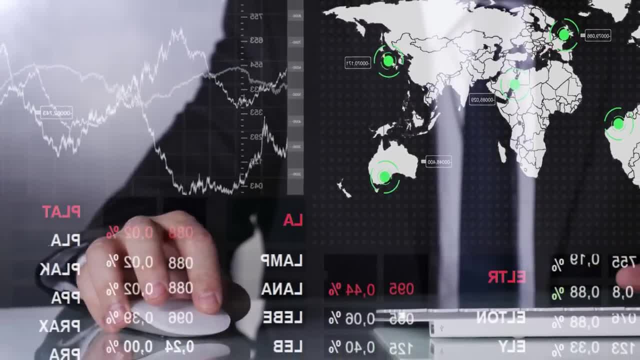 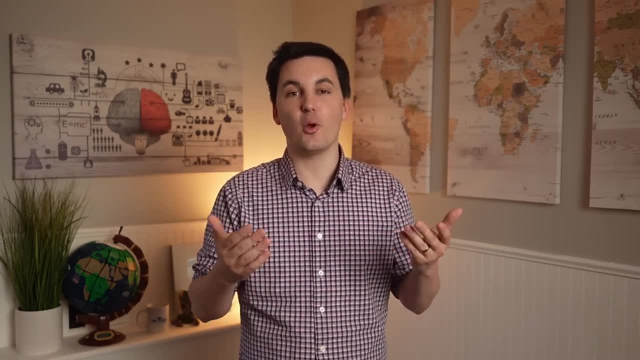 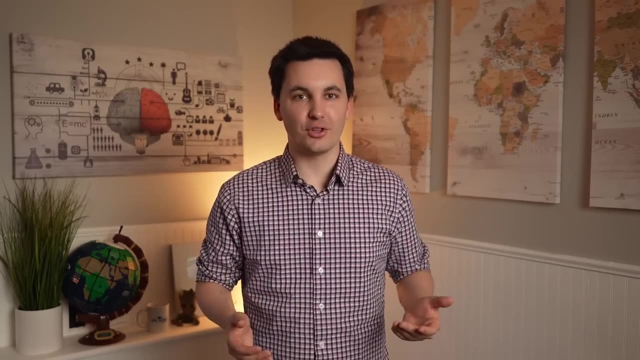 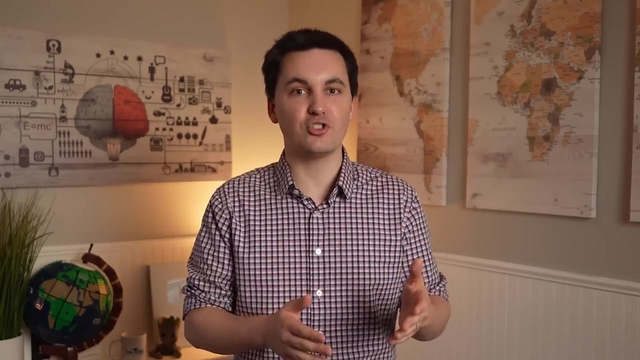 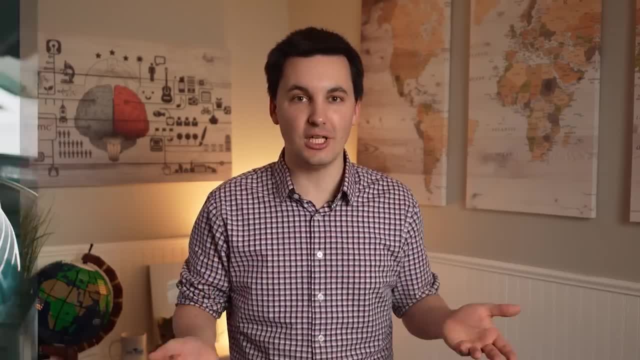 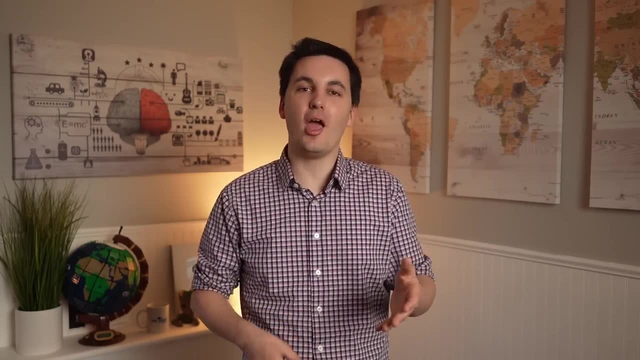 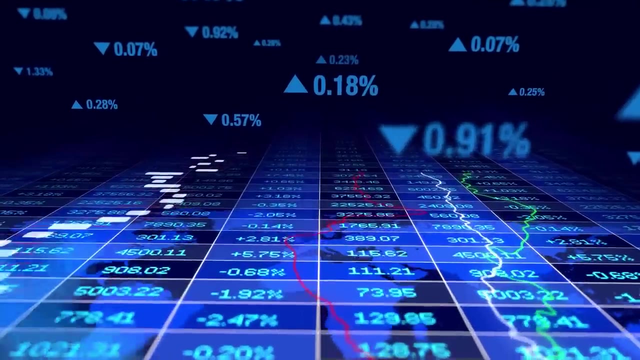 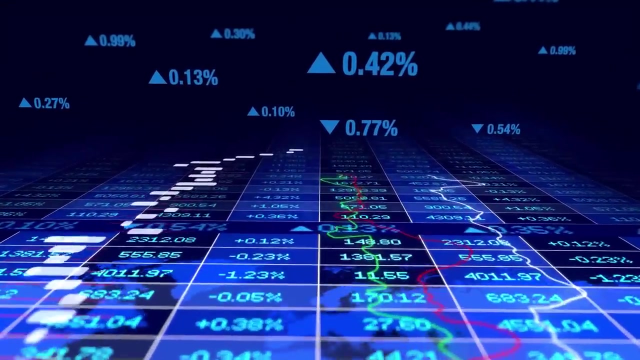 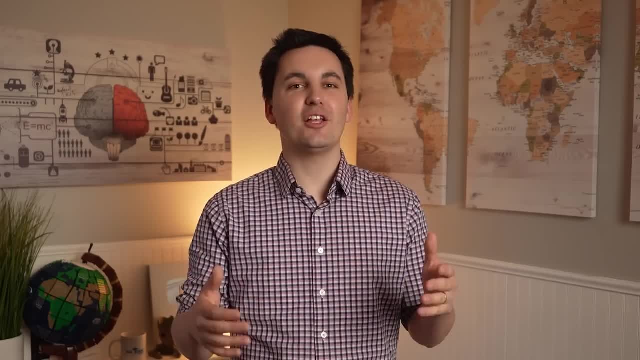 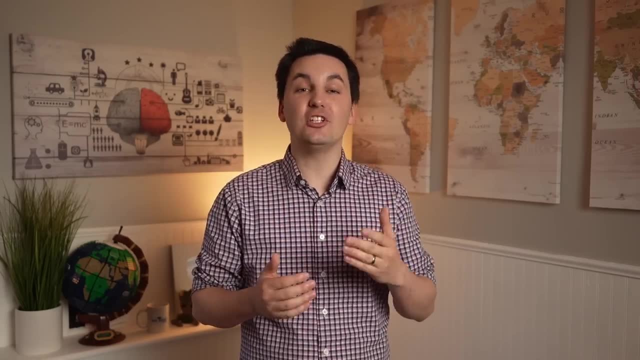 but all levels of a state's economy. For example, we can see that some countries seek to reduce trade and promote domestic production. One way in which this can be accomplished is by implementing tariff. A tariff is a tax or duty imposed by a government. 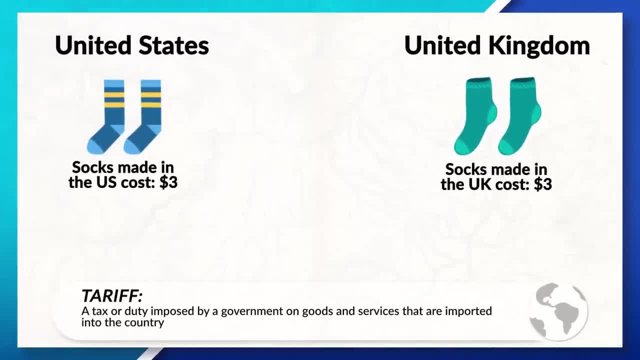 on goods and services that are imported into the country. The goal is to make goods that are produced outside of a country's boundaries more expensive, to ultimately motivate consumers to purchase goods that were made domestically. This happens because the domestic goods do not have the tariff impacting their price. 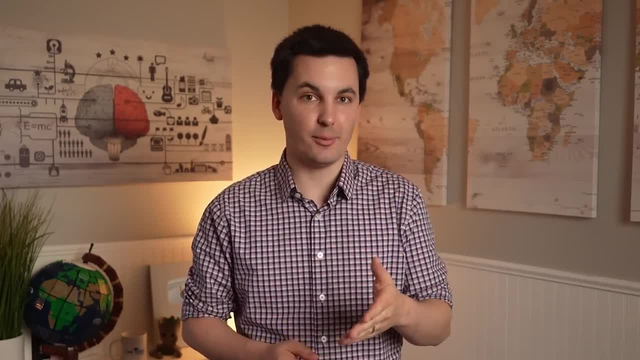 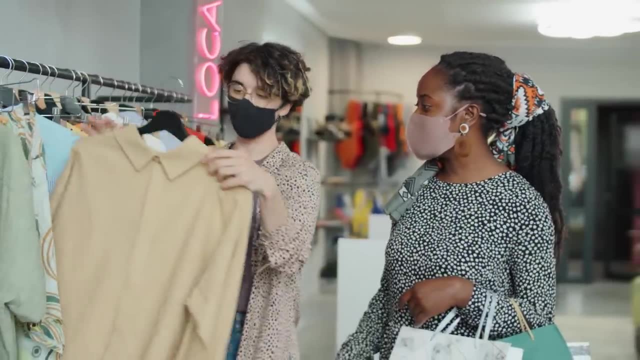 Now it is important to note that the tariff is not paid by the country or government that the tariff is put on. In fact, it's paid by the business. However, we can see that businesses normally pass the extra expenses onto the consumer by raising the price of the product. 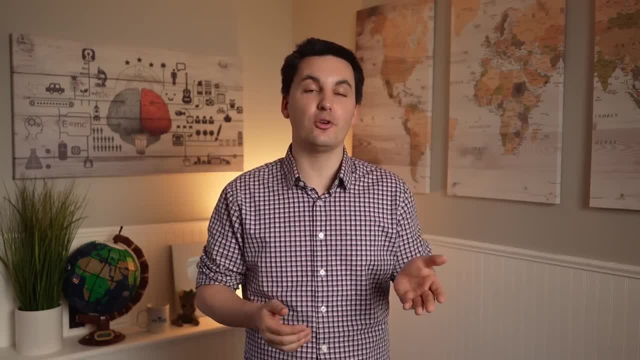 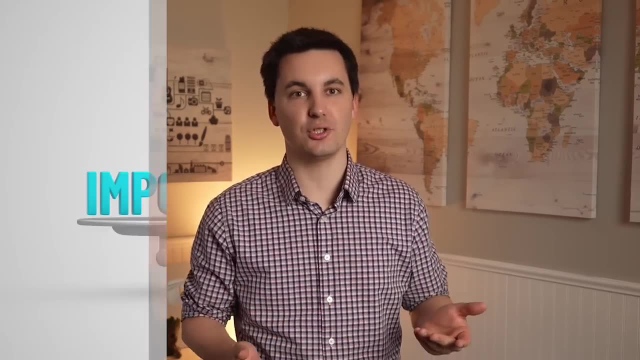 that was impacted by the tariff. So ultimately, the consumer is the one who ends up paying for the tariff. Oftentimes, countries will put tariffs in place if domestic production is more expensive than foreign production or if the country has a trade deficit with another country. 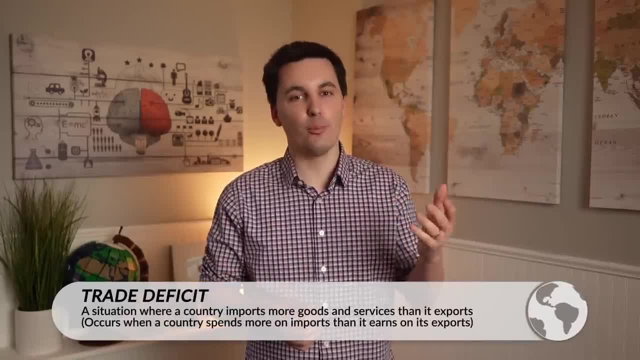 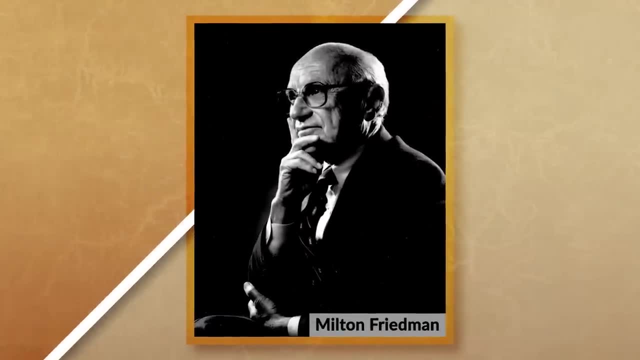 that it wants to reduce. A trade deficit occurs when a country imports more goods and services from another country than it exports. Many economists, such as Milton Friedman, argued that a trade deficit should not be a concern for countries, because countries willingly engage in trade with other countries. 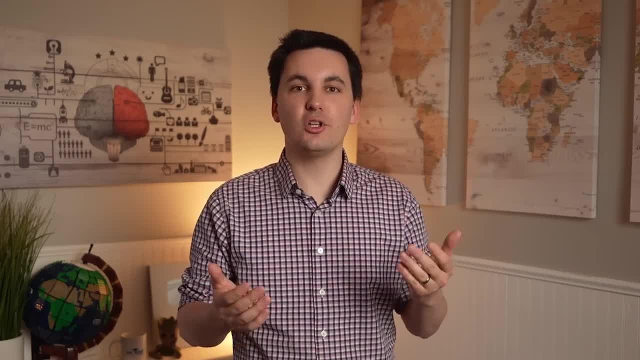 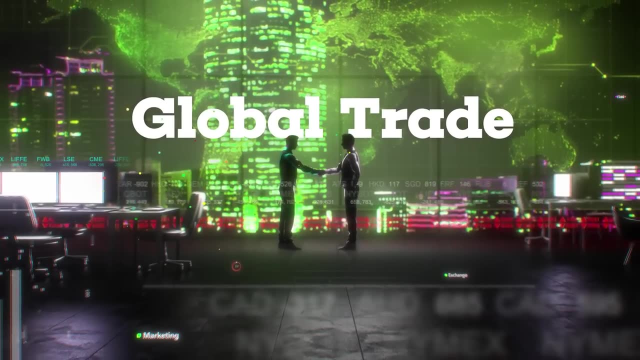 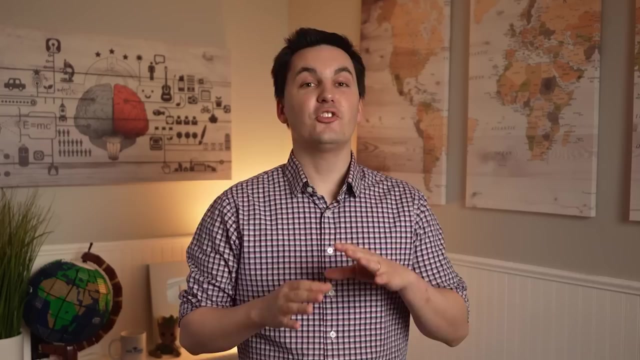 Friedman argued that policies such as tariffs end up distorting the price of the market and prevent the market from efficiently using its resources. Friedman believed that it was better for countries to increase trade with other countries to allow for free market competition, which would result in economic prosperity. 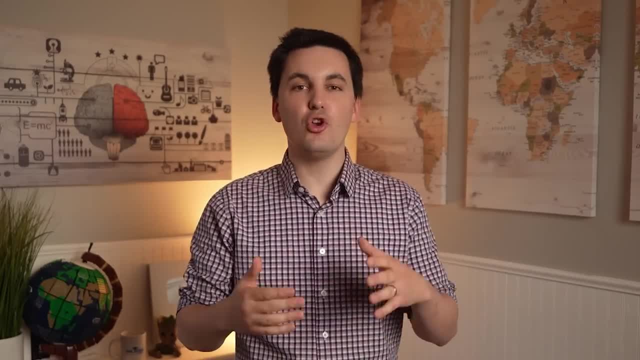 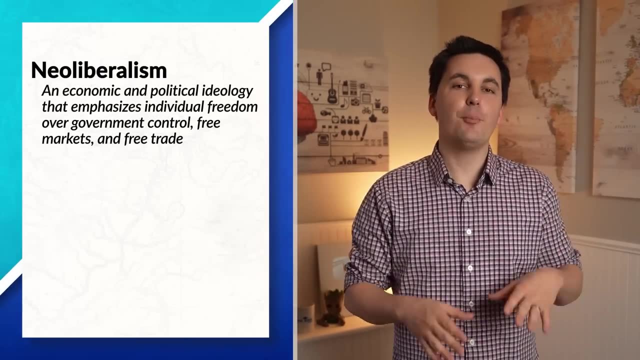 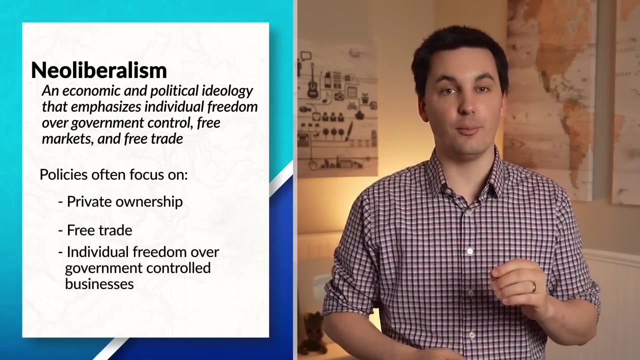 This idea of promoting free trade and increasing global trade is known as neoliberalism, which is characterized by policies that seek to reduce the amount of government intervention in the economy and promote free market capitalism. These policies often focus on private ownership, free trade and individual freedom. 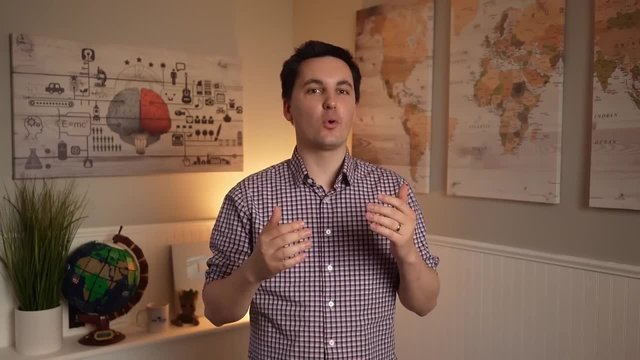 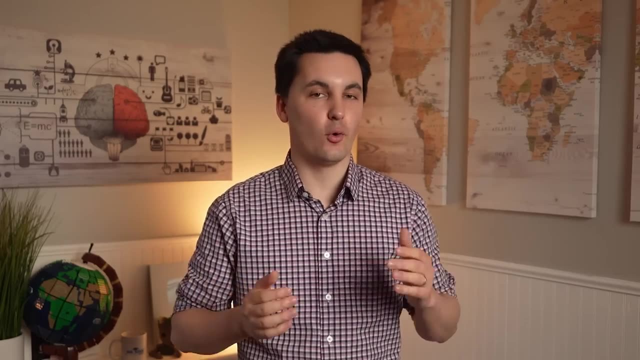 over government-controlled businesses. When looking at the world today, we can see a variety of different organizations and trade deals which are based off of neoliberal policies. Organizations such as the World Trade Organization have been created to try and promote globalization and free trade around the world. 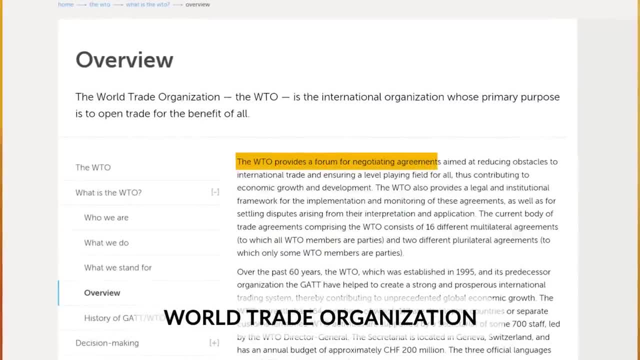 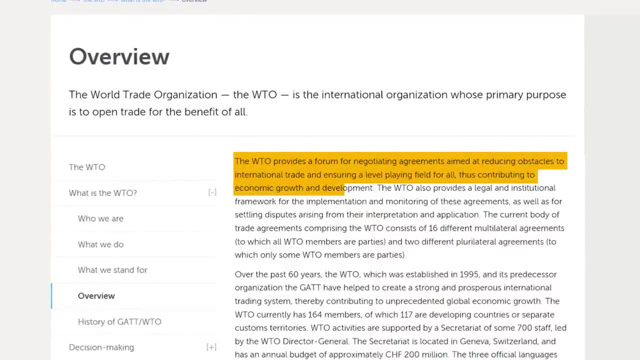 The World Trade Organization provides a forum for negotiating agreements aimed at reducing obstacles to international trade and ensuring a level playing field for all, Thus contributing to economic growth and development. The primary purpose of the organization is to open trade for the benefit of all. 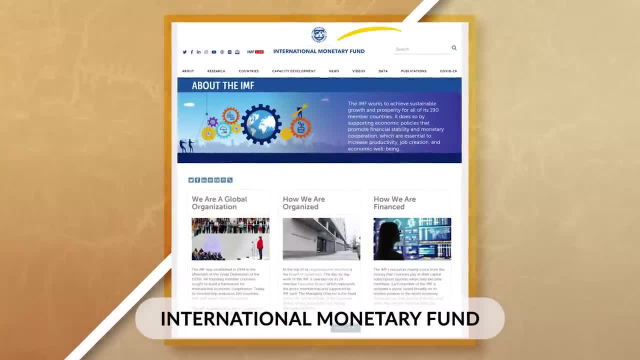 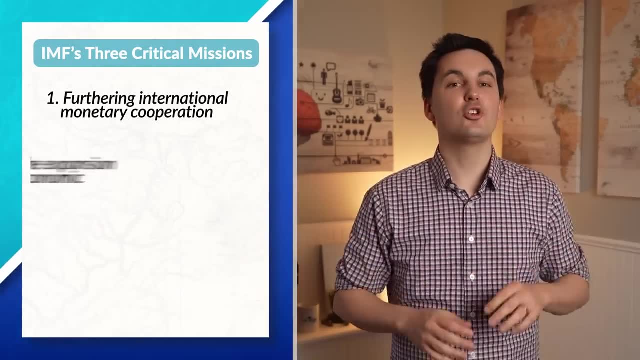 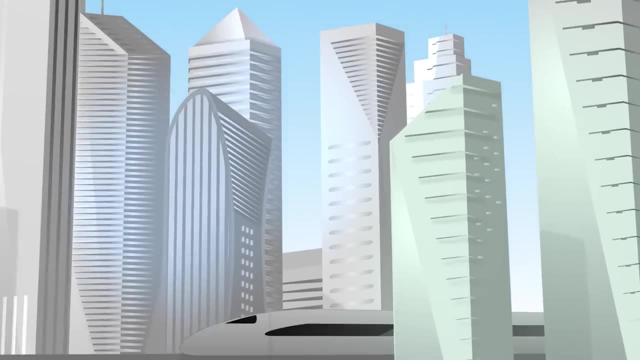 Another organization we can look at is the impact monetary fund has had on the global market. The IMF has three critical missions: Furthering international monetary cooperation, encouraging the expansion of trade and economic growth and discouraging policies that would harm prosperity. These missions all connect back to the idea of promoting 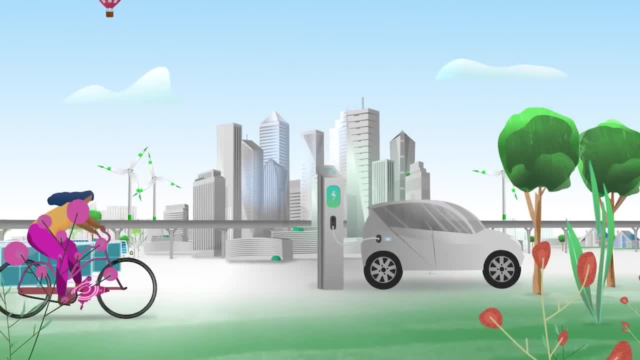 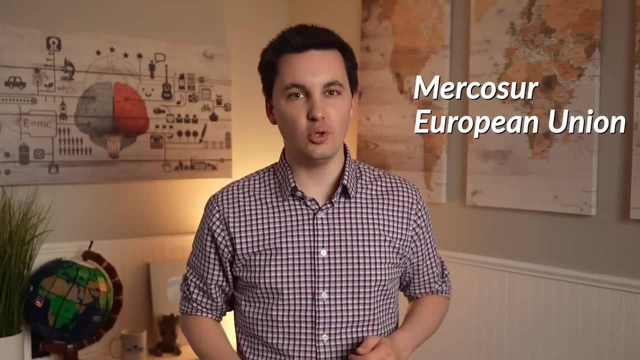 sustainable economic growth for countries around the world through trade and commerce. We can also look at other organizations that promote globalization, such as MERCOSUR, the European Union and OPEC, just to name a few. MERCOSUR consists of different countries in South America, with its main. 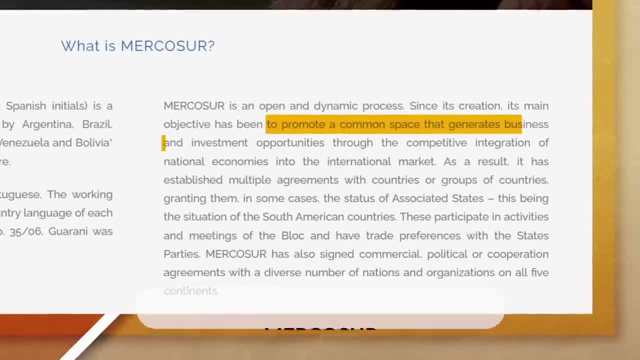 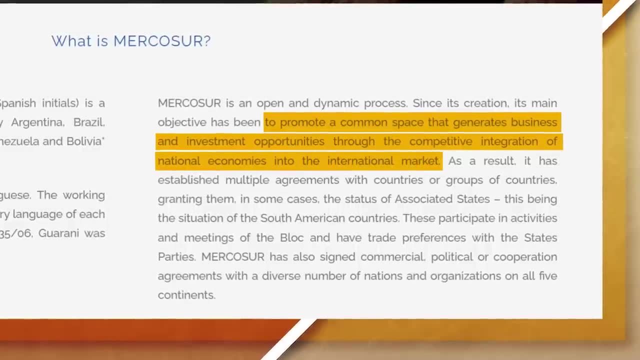 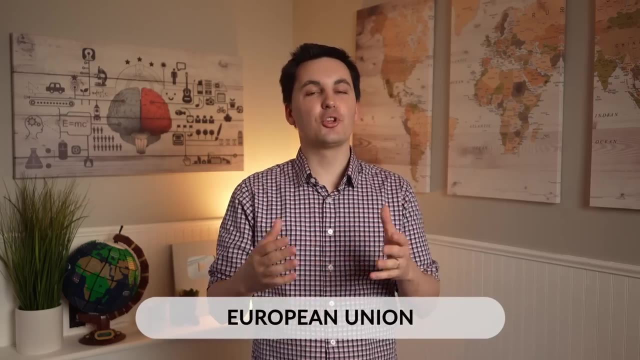 objective being to promote a common space that generates business and investment opportunities through competitive integration of national economies into the international market. The European Union is a political and economic union of states primarily located in Europe. It was created with the goal of promoting peace, stability and economic prosperity in the region. 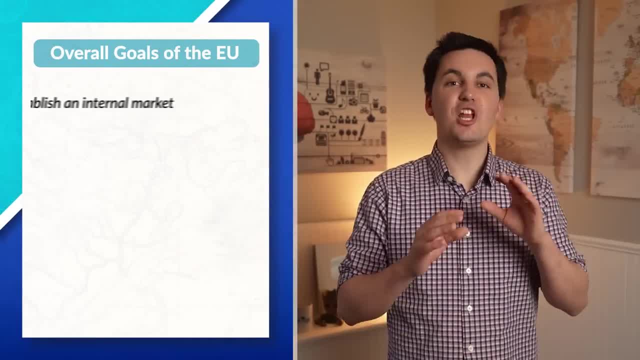 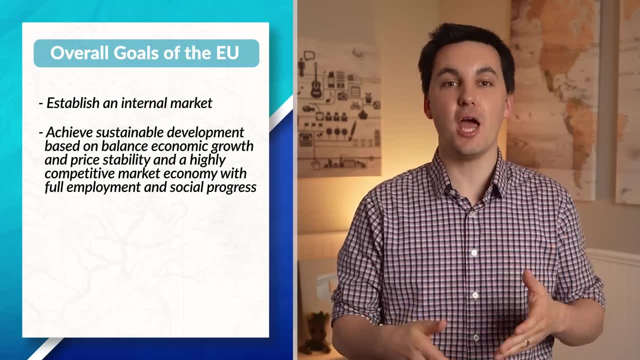 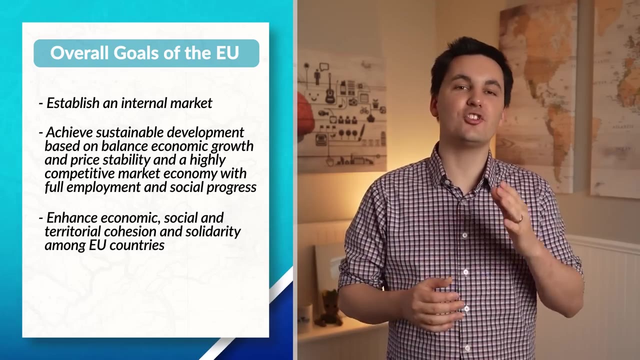 Today, some of the European Union's overall goals are to establish and internal market. achieve sustainable development based on balanced economic growth and price stability and a highly competitive market economy with full employment and social progress. enhance economic, social and territorial cohesion and solidarity among EU countries. and establish an economic and monetary union. 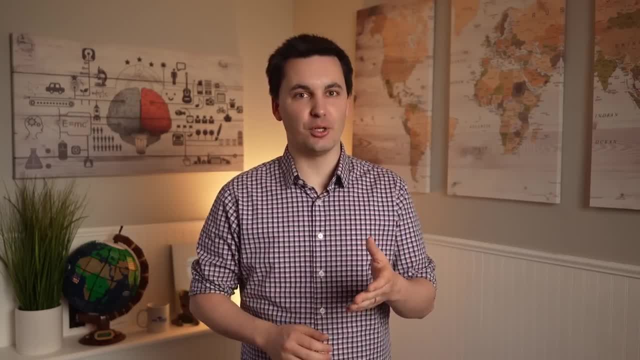 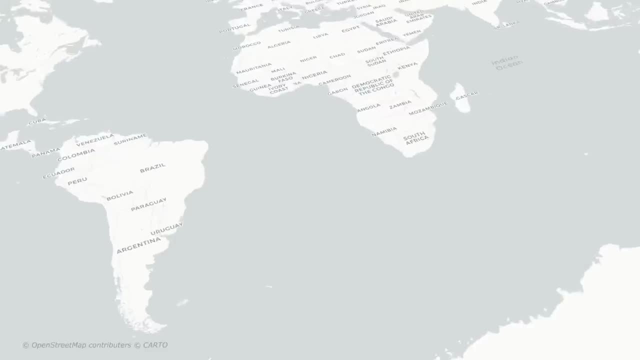 whose currency is the euro. There are many other goals of the organization, but overall we can see a focus to increase trade and commerce between members, to promote economic growth for countries and to promote economic development for the world. The last organization I wanted to mention was OPEC, which is a little bit. 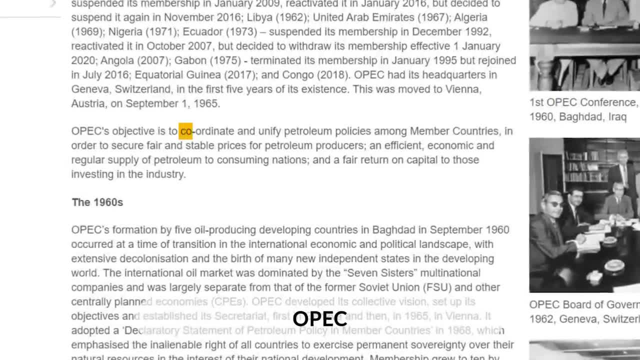 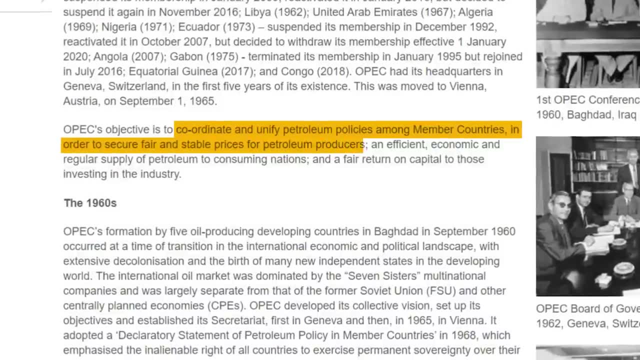 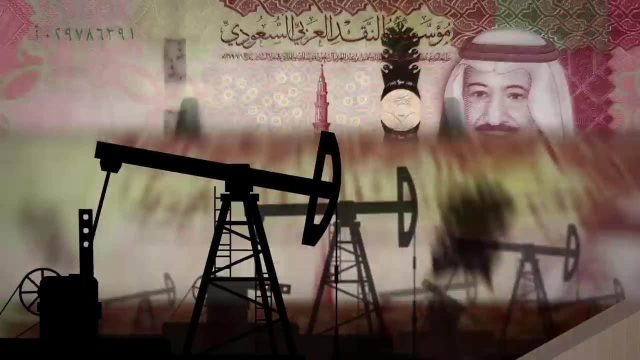 more controversial. We can see that OPEC's objective is to coordinate and unify petroleum policies among member countries in order to secure fair and stable prices for petroleum producers. On one hand, we can see how OPEC goes against a free market system and competition by using its control over 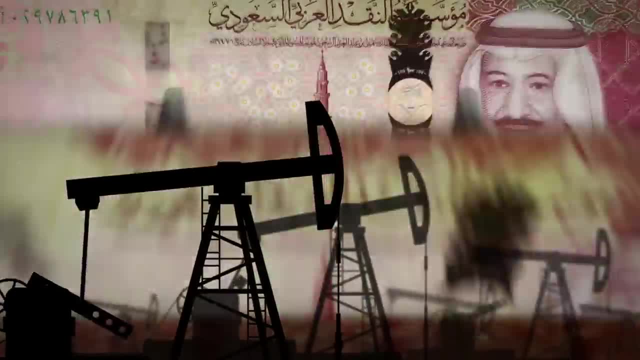 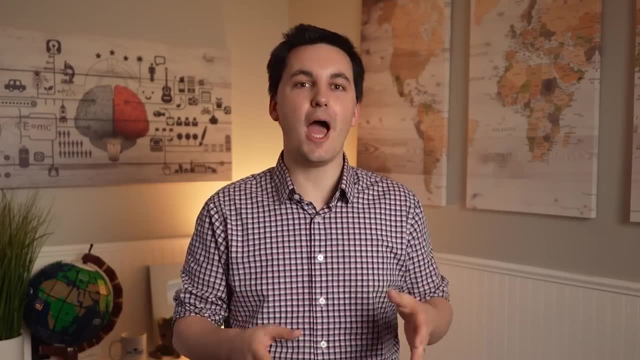 oil production to influence the global supply of oil and, ultimately, the price of oil, which restricts competition and can artificially influence inflation. But, on the other hand, we could also see aspects of OPEC that do promote neoliberal policies, such as efficiently using resources, allowing for 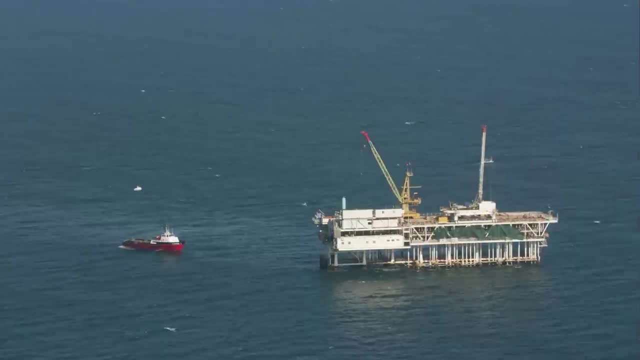 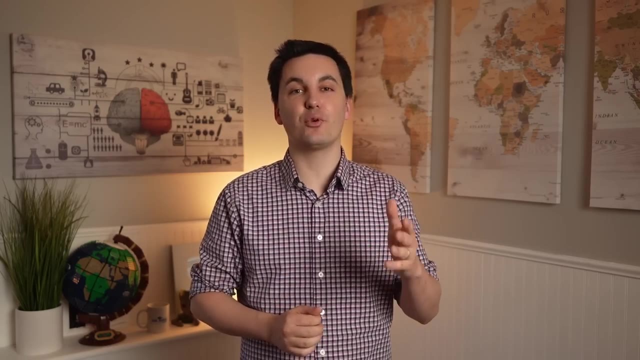 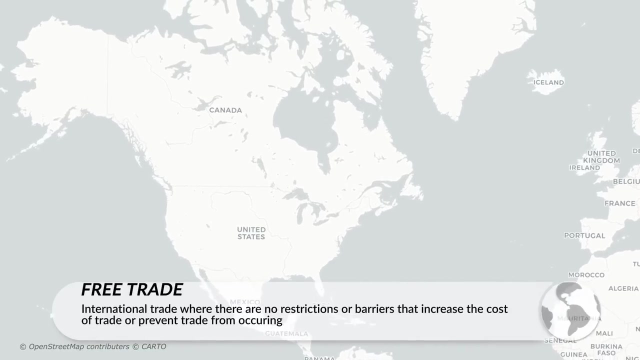 stabilization to occur in oil prices and by promoting stable economic growth for all oil producing countries in the organization. Neoliberal policies have also led to the creation of free trade agreements such as NAFTA, which was replaced by the USMCA in 2020.. The goal here is to bring free trade between: 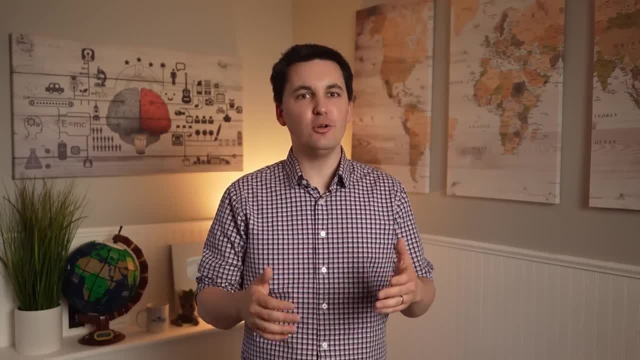 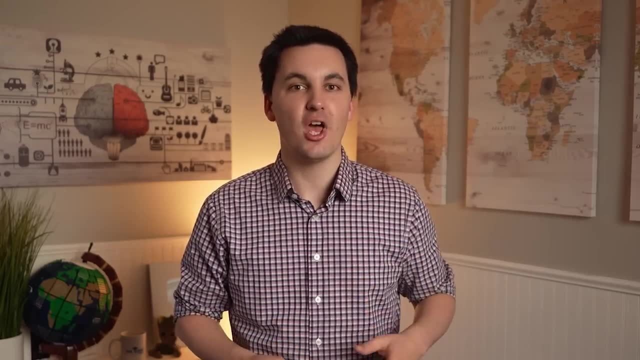 countries in the region. At the end of the day, we can see how neoliberal policies have encouraged the development of global trade networks and have led to the creation of new spatial connections between countries and regions around the world. Now, just like everything else we've talked about, there is negative 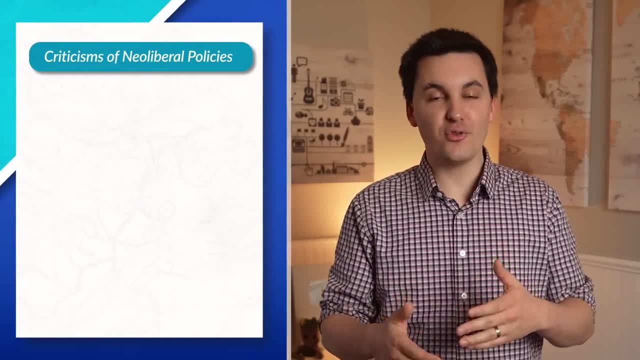 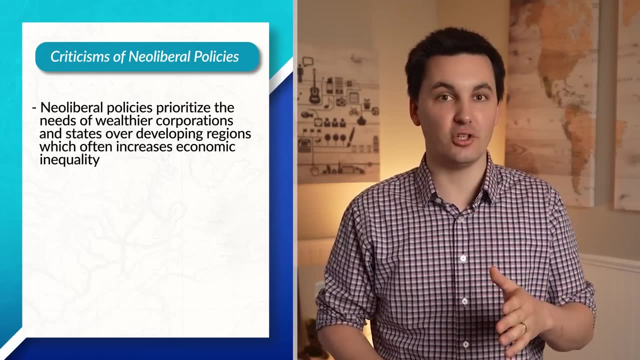 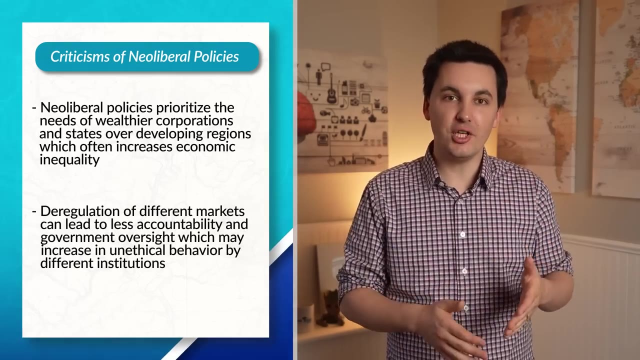 aspects to neoliberal policies as well. Critics have pointed out that oftentimes, neoliberal policies prioritize the needs of wealthier corporations and states over the developing regions, which often increases economic inequality- inequality around the world. Deregulation of different markets can also lead to. 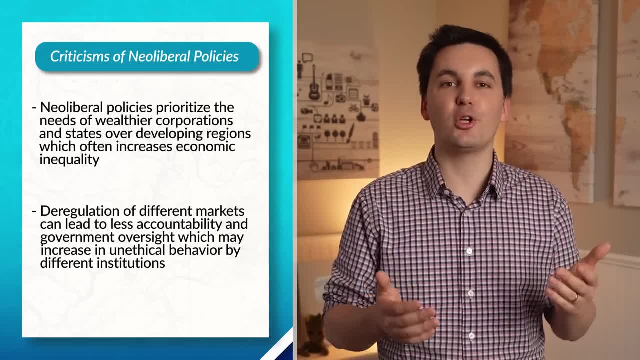 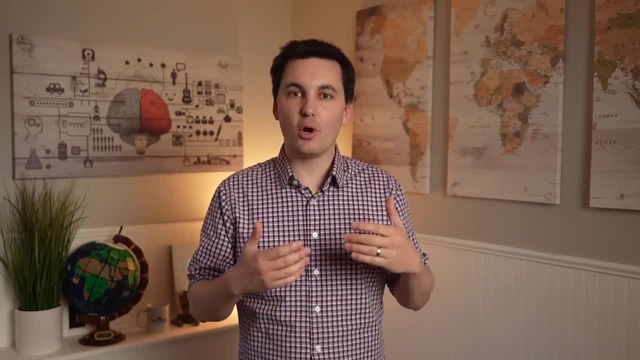 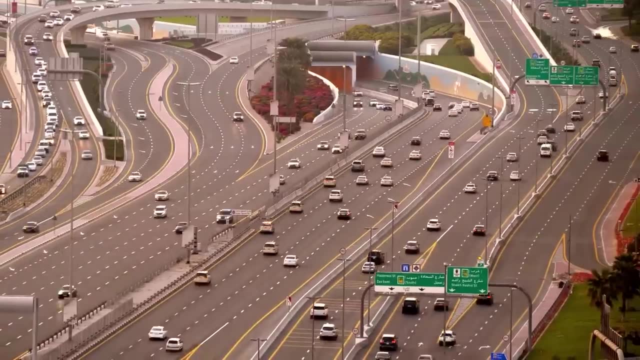 less accountability and government oversight, which may increase unethical behavior by different institutions. These policies could also negatively impact the stability of developing nations, as they now are competing with states whose economies are more advanced and are made up with more advanced, robust technology and infrastructure. These policies could also hurt workers in more economically. 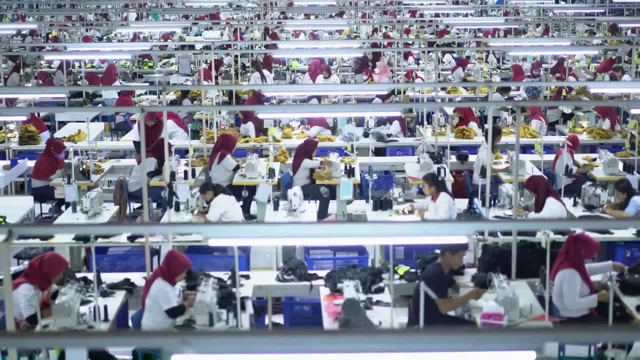 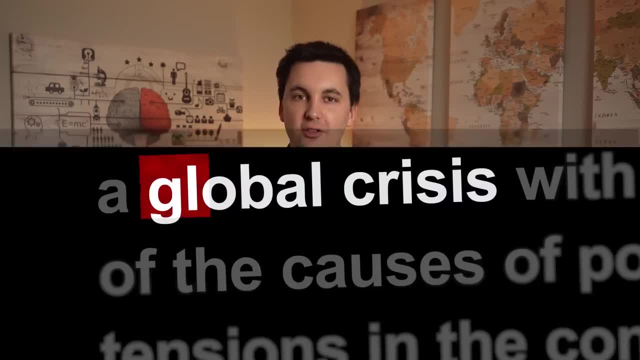 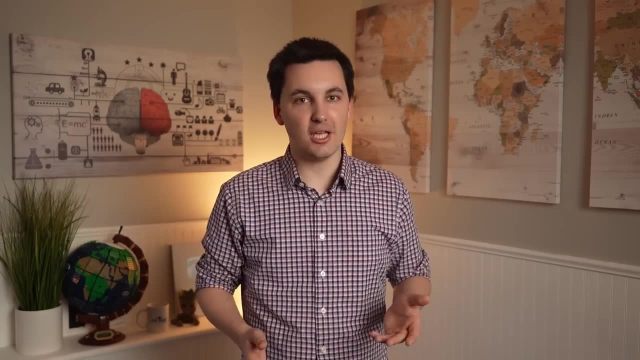 advanced regions, as they now have to compete with workers in less economic and economically developed areas, which often work at a much cheaper rate. Now, a connected global community also means that crises in one part of the world will have a ripple effect on the larger global community. Such was the case in 2008, when the financial 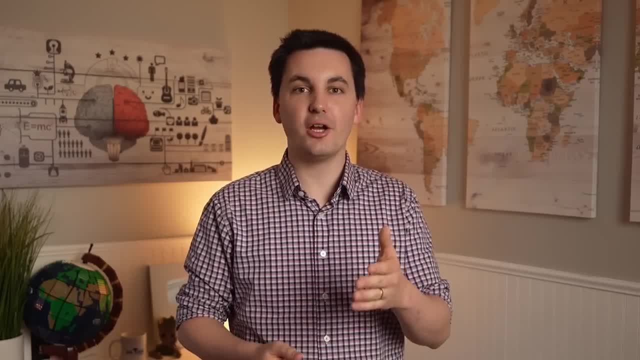 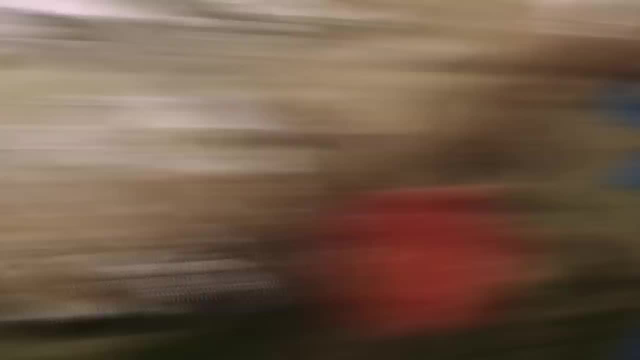 market collapsed in the United States, which ended up impacting the entire global community for years to come. Or we could look at another example, such as COVID-19,, which resulted in the global economy grinding to a halt, resulting in mass shortages and broken supply chains around the 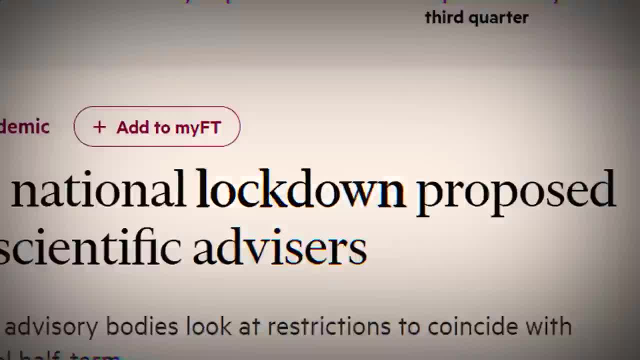 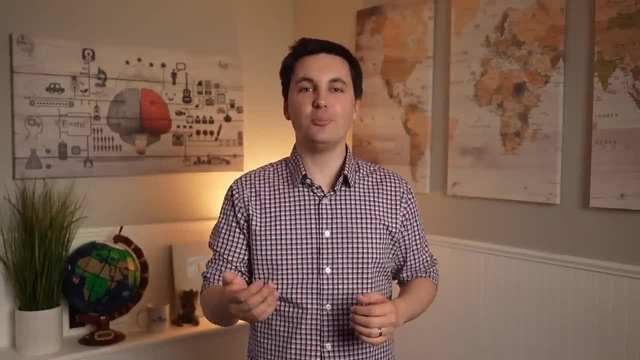 world, all of which left governments scrambling to pivot to protect their citizens and keep their economies from collapsing. Speaking of supply chains, we can also look at how the global economy can be impacted by something as simple as a blocked canal, which we saw in May 2021,. 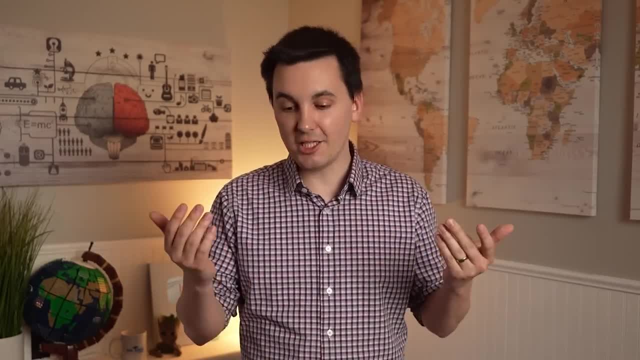 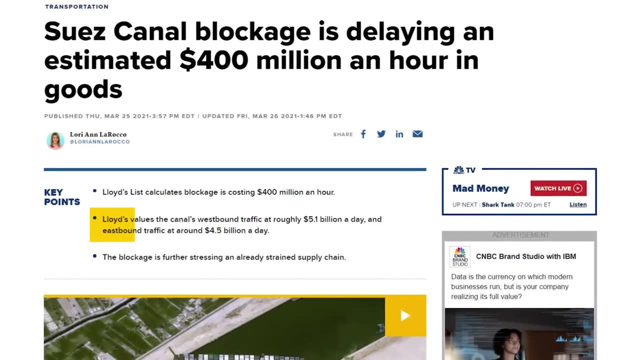 when the Ever Given ran aground in the Suez Canal, blocking access to the canal. This canal is one of the busiest trade routes in the world and the blocking of the canal was estimated to cost around $9.6 billion in trade a day, which we could break down to $400 million. 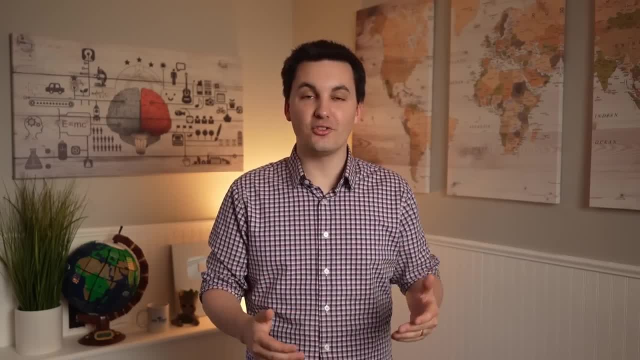 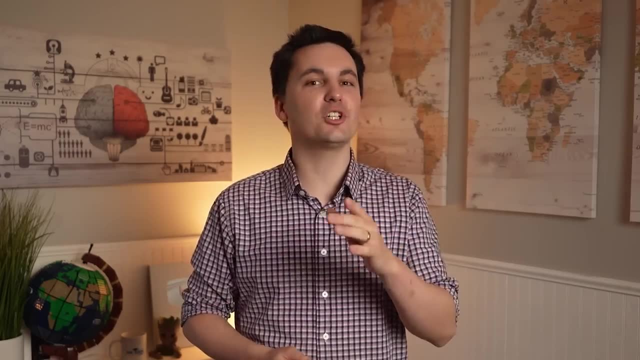 an hour, So we can see that when problems do arise in the global economy, the consequences can be quite significant. So what do you think? Do the benefits outweigh the negatives? Let me know in the comment section down below. One thing is for sure, though, as time goes on: 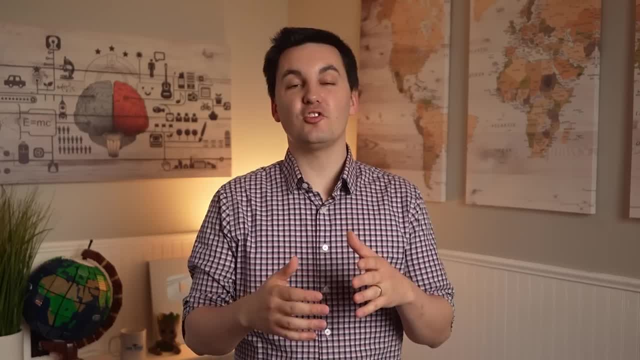 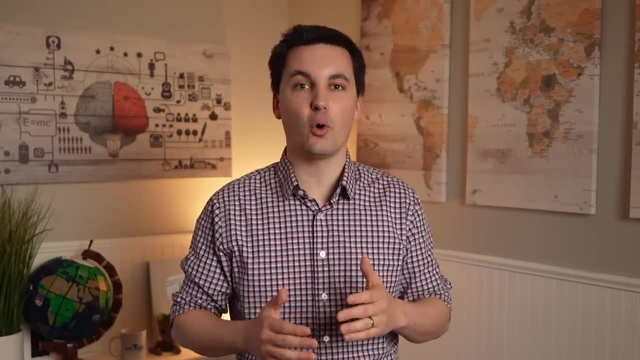 countries will only continue to become more interdependent. Organizations such as the International Monetary Fund and the World Bank continue to work to promote economic development around the world. This often happens through microlending, resulting in more economies becoming closely connected, and even more so in the global economy. So what do you think? Do you? 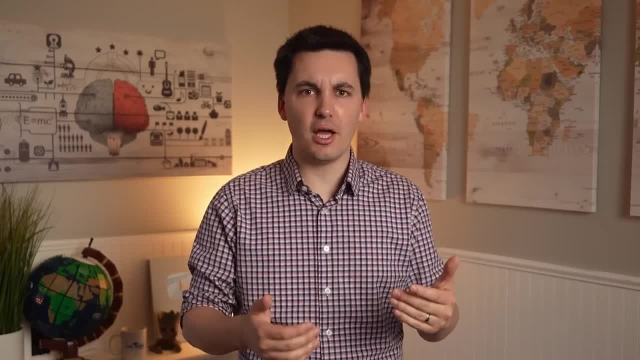 think this is a good thing. Let me know in the comment section down below. At the end of the day, we can see that every level of society is impacted by our global community. At the local scale, workers now compete with a global workforce. 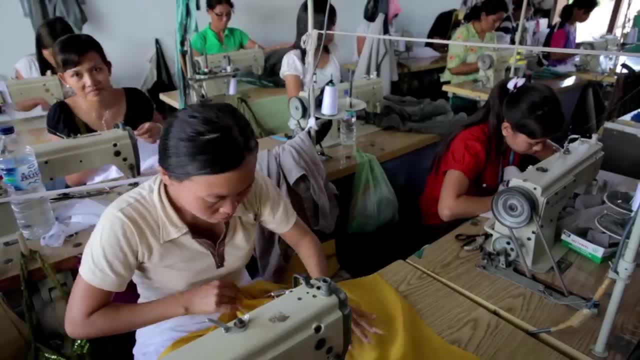 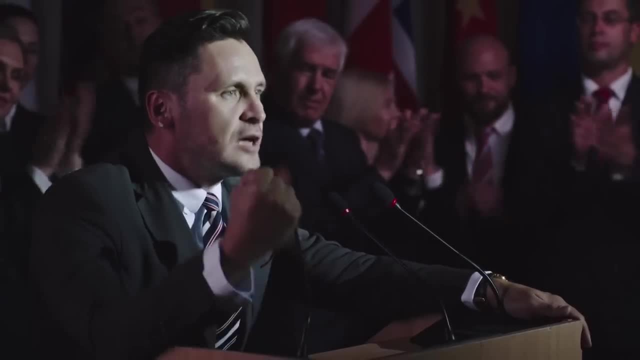 which leads to a more productive workforce but also means the loss of jobs, as businesses relocate work to cheaper labor markets. At the national scale, we can see the impact that government policies have not only on the price of goods but the availability of those.